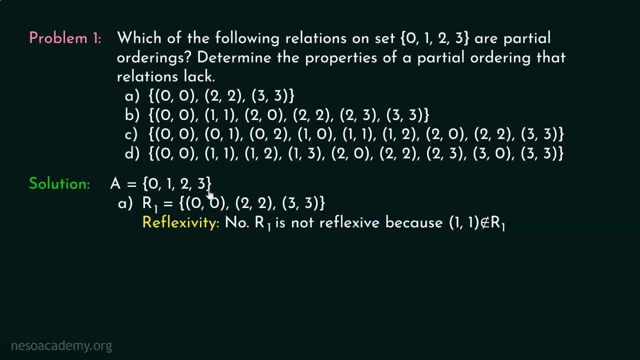 We have total four elements in this set A. For every element we must have the ordered pair A, A in R1.. But in this relation we do not have an ordered pair 1, 1.. Therefore this relation is not reflexive. 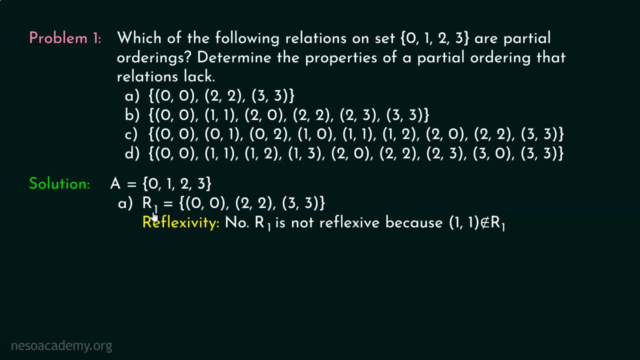 Right, Let's check whether this relation is antisymmetric or not. Obviously, this relation is antisymmetric because if A- B belongs to R1 and B- A belongs to R1, then A is equal to B. We have all the ordered pairs of the form A- A. 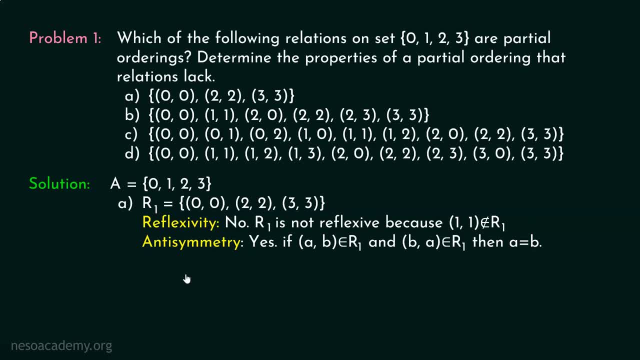 Therefore, this relation is antisymmetric. Apart from this, this relation is transitive as well. It is quite trivial. Therefore, R1 is not a partial order, because reflexive property is not satisfied for this relation. Right Now, let's see: 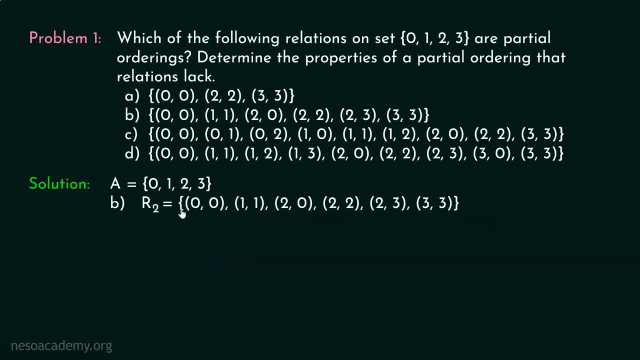 Is this relation a partial order or not? Let's say, this relation is R2.. This relation is reflexive because we have ordered pairs 0, 0, 1, 1, 2, 2 and 3, 3 in this relation. 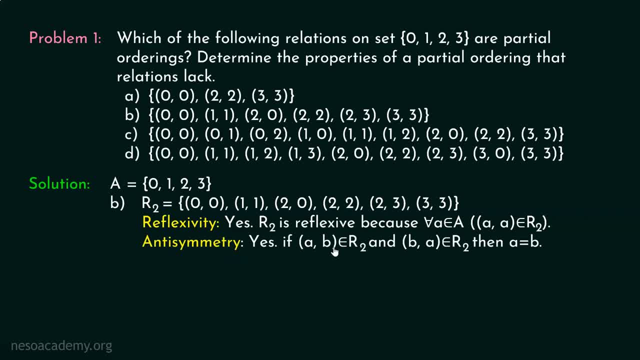 This relation is antisymmetric as well, because if A- B belongs to R2 and B- A belongs to R2, then A is equal to B. We have ordered pairs 0, 0,, 1, 1,, 2,, 2, 3, 3.. 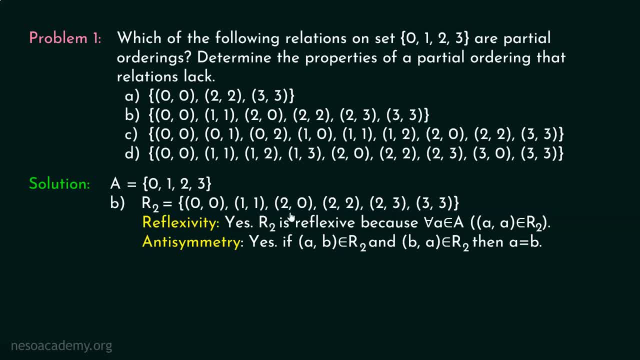 Apart from this, we have these two ordered pairs: 2, 0 and 2, 3.. You can see that 2, 0 is there in this relation, but 0, 2 is not there in this relation. We have 2, 3,, but we do not have 3, 2 in this relation. 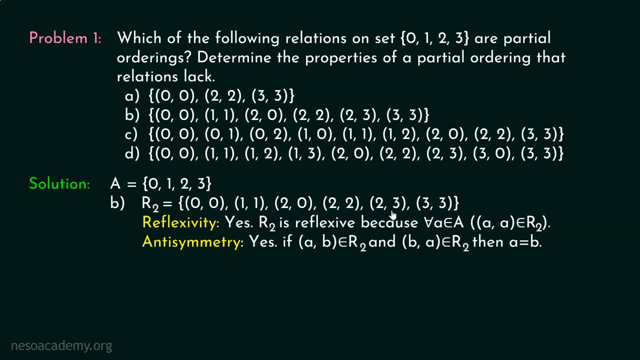 Therefore, this relation is antisymmetric. Apart from this, this relation is transitive as well. You can check this on your own. All the three properties are satisfied. Therefore, we can say R2 is a partial order. Right Now let's see whether this relation is a partial order or not. 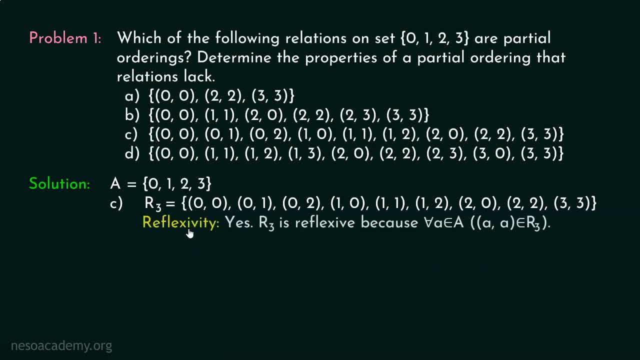 Let's name this as R3.. This relation is reflexive because we have 0, 0,, 1,, 1,, 2,, 2 and 3, 3.. This relation is reflexive because we have 0, 0, 1,, 1,, 2,, 2 and 3, 3.. 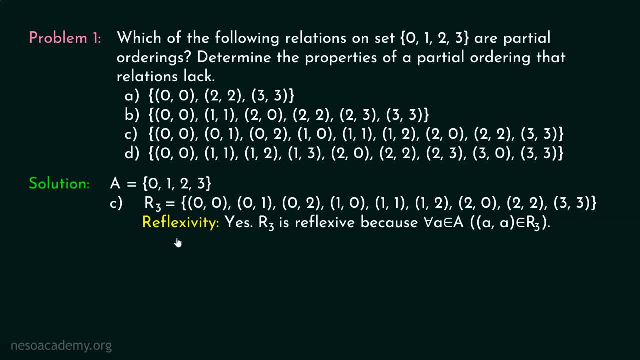 This relation is reflexive because we have 0,, 0,, 1,, 1,, 2,, 2 and 3, 3.. Apart from this, please note that this relation is not antisymmetric. Apart from this, please note that this relation is not antisymmetric. 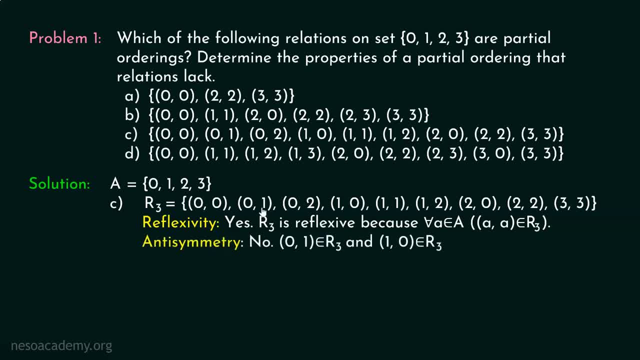 Apart from this, please note that this relation is not antisymmetric, Because we have 0, 1 in this relation and 1, 0 at the same time. Because we have 0, 1 in this relation and 1, 0 at the same time. 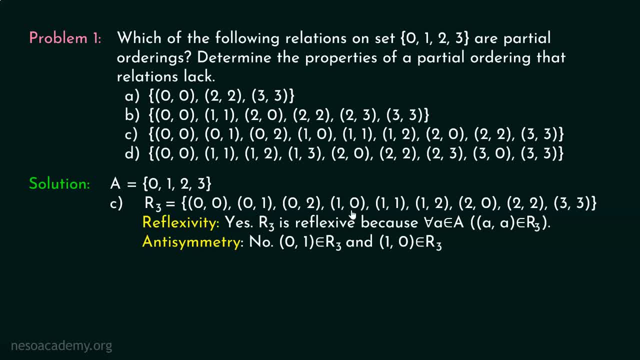 Because we have 0, 1 in this relation and 1, 0 at the same time. Therefore, this relation is not antisymmetric. Therefore, this relation is not antisymmetric, Right, And yes, this relation is not transitive as well. 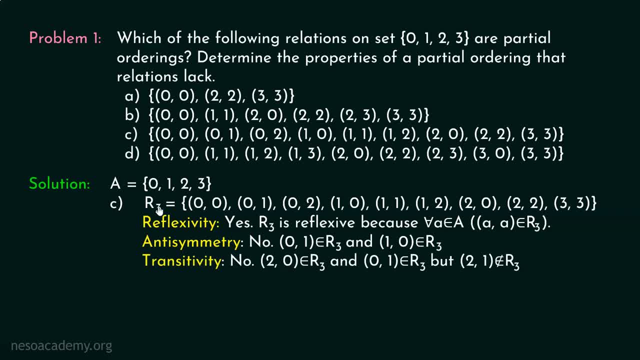 We have 2, 0 in this relation R3.. We have 2, 0 in this relation R3.. You can see over here: 2, 0 is there in R3.. We have 0, 1 in this relation. 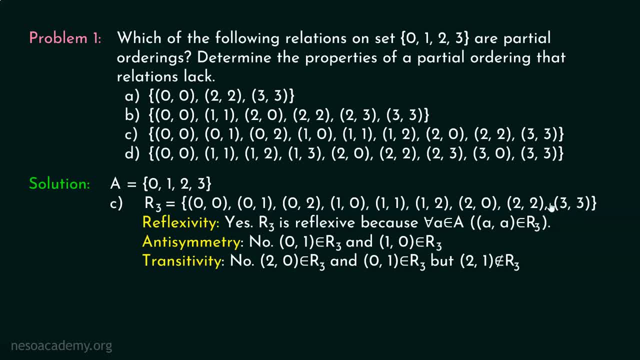 but we do not have 2, 1 in this relation. but we do not have 2, 1 in this relation. We have 2, 0, 0, 1, but we do not have 2, 1.. 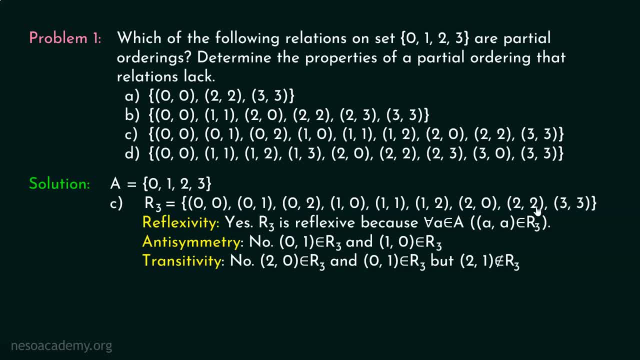 We have 2, 0,, 0, 1,, but we do not have 2, 1.. Therefore, it is clear that this relation is not transitive. Therefore, it is clear that this relation is not transitive. 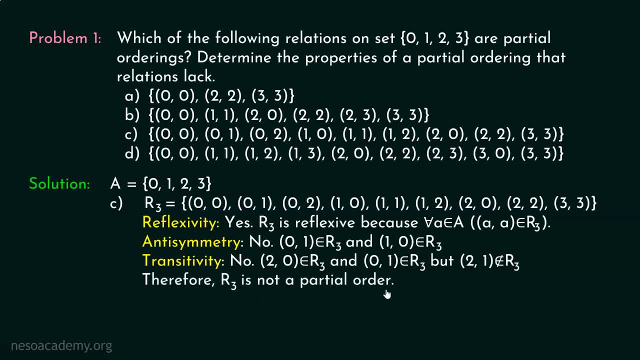 Therefore, we can say that this relation is not a partial order. Therefore, we can say that this relation is not a partial order. R3 is not a partial order. R3 is not a partial order. Let's say this relation is R4. 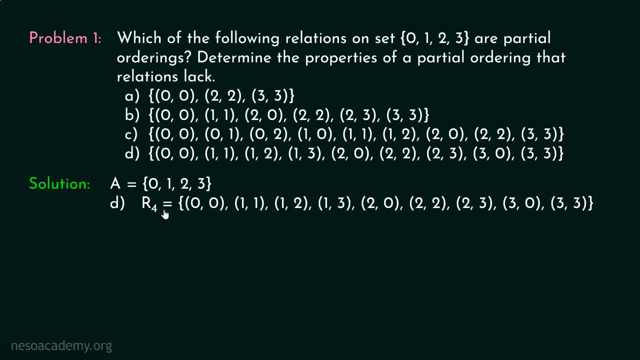 and let's see whether this relation is a partial order or not. and let's see whether this relation is a partial order or not. Let's first check the reflexive property. Yes, this relation is reflexive because it has 2, 0, 1, 1, 2, 2. 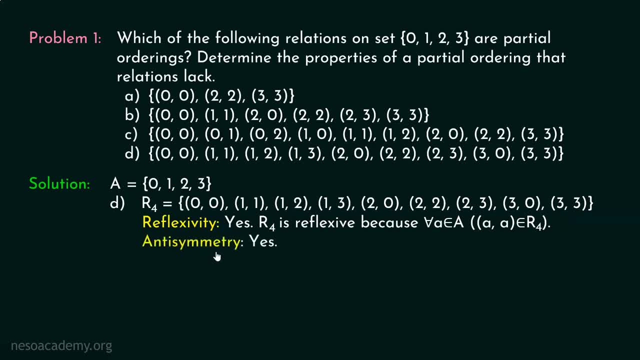 and 3, 3 in this relation. This relation is antisymmetric also, and you can check this. We have 2, 2 in this relation, but we do not have 2,1.. We have 1, 3, but we do not have 3,1. 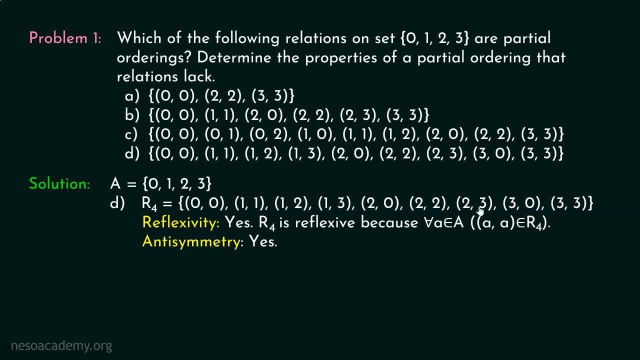 We have 2, 0,, but we do not have 0, 2.. We have 2, 3,, but we do not have 3,2.. We have 3,0,, but we do not have 0,3.. 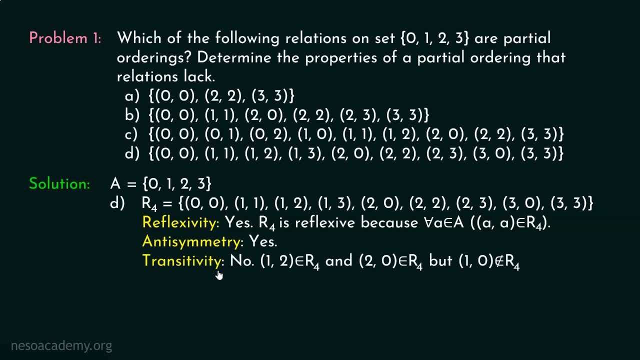 Therefore, this relation is antisymmetric. Apart from this, this relation is not transitive. Why, in this relation, we have 2: 0 in this relation, but we do not have 1: 0 in this relation, Right? So it is clear. 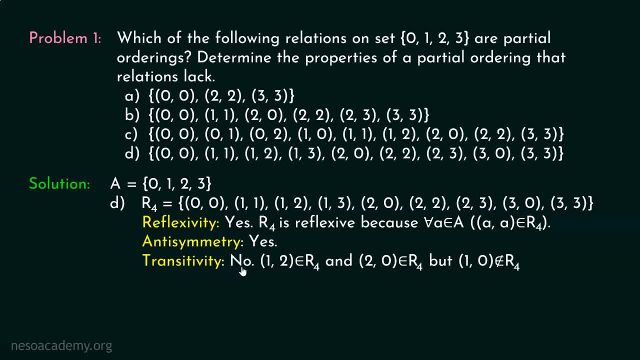 that this relation is not transitive, Because transitivity is not satisfied. so we can say that this relation is not a partial order. Right Now let's discuss problem 2.. Let's say S is the set of all people in the world and R is the relation. 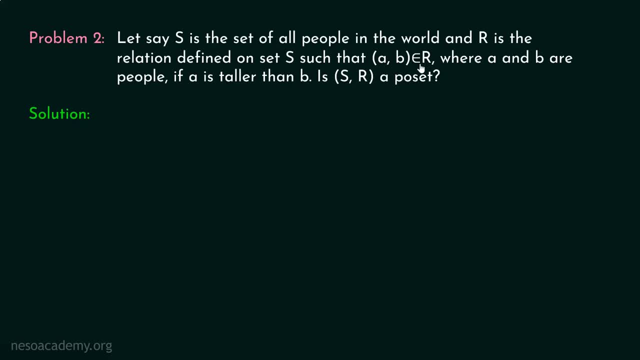 defined on set S, such that A, B belongs to R, where A and B are people. if A is taller than B, Now is S R opposite. This is the question. Okay, We have relation R which consists of all ordered. 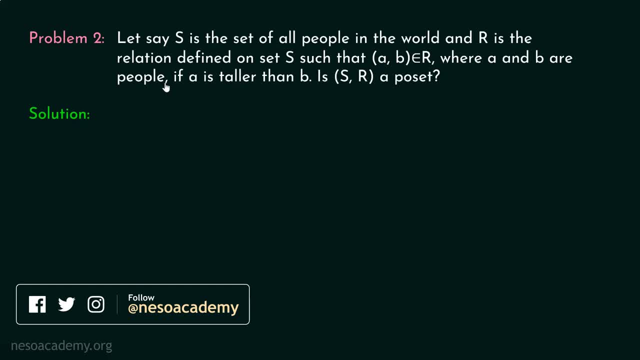 pairs of the form A- B, where A and B are people and A is taller than B. Okay, Apart from this, this relation is defined on the set of all people in the world, Right. So we have relation R, which consists of: 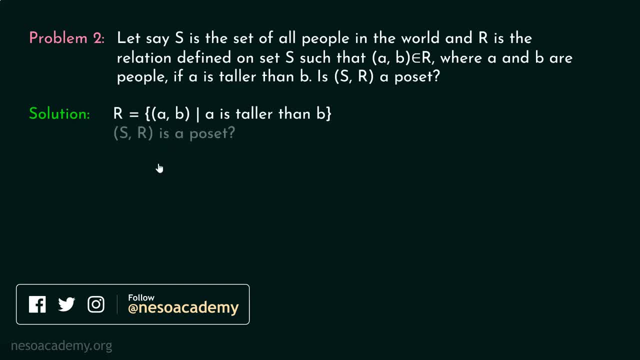 ordered pairs A- B, such that A is taller than B, And we have to identify whether S- R is a posit or not. This relation, R, is defined on set S, which consists of all people in the world. We have to identify whether S. 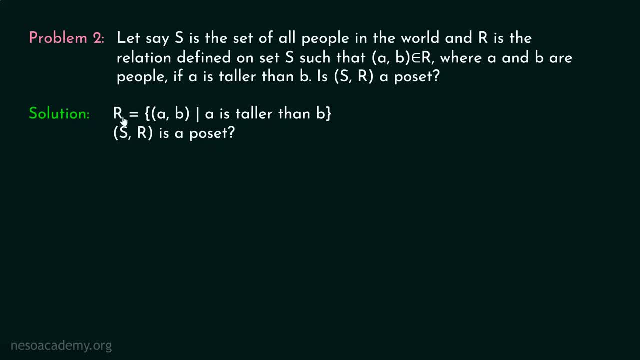 R is a posit or not. For this we will check whether this relation is a partial order or not. Right, Obviously, we must check the reflexive property first For all. A belongs to S A. A must belong to R. 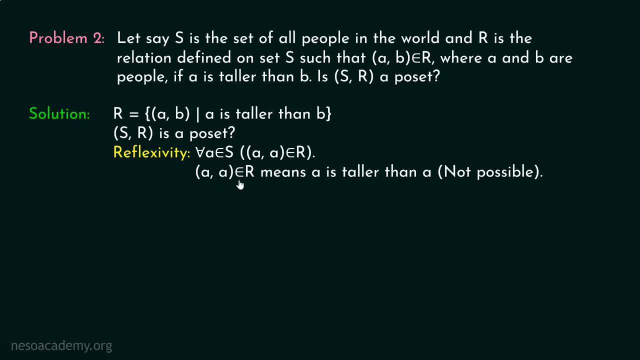 A is not taller than A Right A. A does not belong to R. How is it possible that A is taller than A Right? Therefore, R is not reflexive. Let's see the antisymmetric property. We know that according. 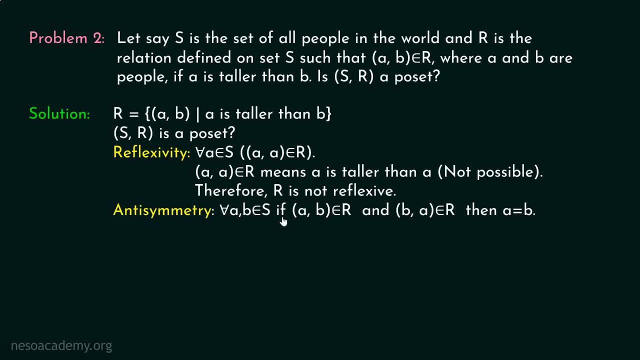 to antisymmetry for all. A- B belong to S. if A- B belongs to R and B A belongs to R, then A is equal to B. Now what does this statement mean If A is taller than B? 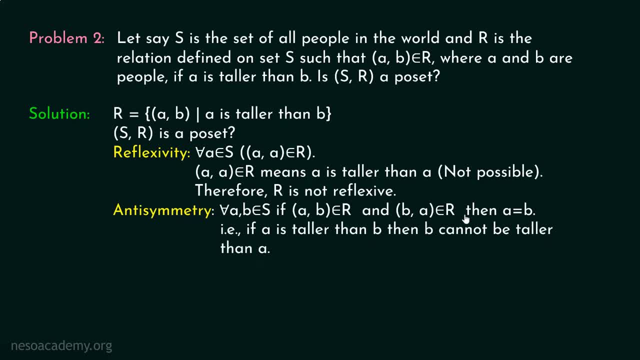 then B cannot be taller than A. That is what this statement is saying, Right? If A is taller than B, then B cannot be taller than A. Obviously, this is true. Therefore, we can say that this relation is antisymmetric. 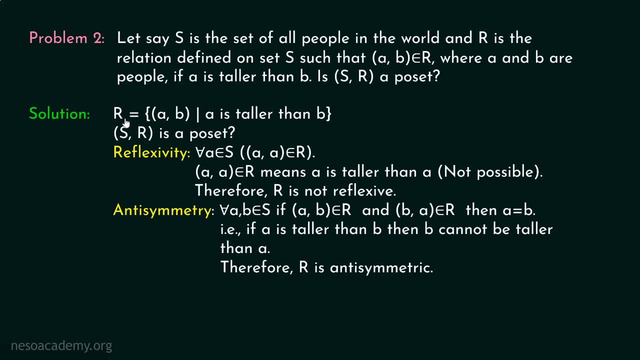 Let's see whether transitive property is satisfied for this relation or not. Yes, of course this relation is transitive. If A is taller than B and B is taller than C, then obviously A is taller than C. There is no doubt about this. Therefore, 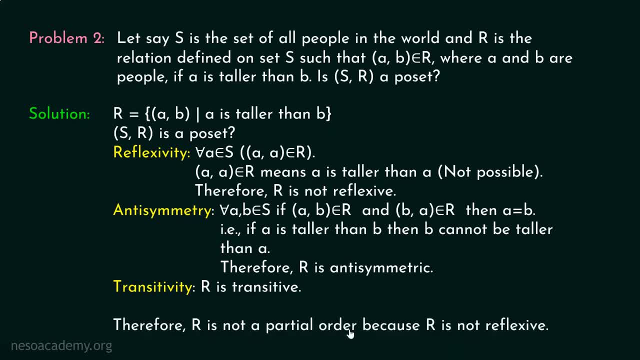 we can say that R is not a partial order because R is not reflexive. It must be well noted that R is not reflexive, Therefore this relation is not a partial order and hence S R is not opposite. Right Now let's see problem 3.. 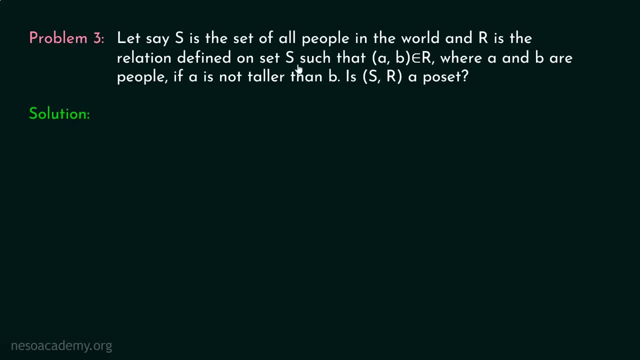 Let's say S is a set of all people in the world and R is the relation defined on set S, such that A- B belong to R, where A and B are people, if A is not taller than B Instead of A is taller than B. now we have 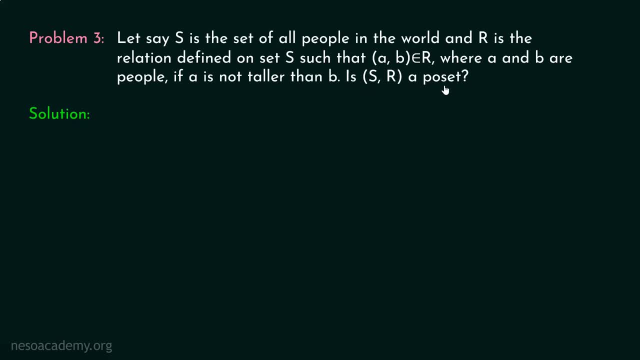 A is not taller than B? Is S R opposite? Let's identify. We are available with this relation, that is, a set of all ordered pairs A- B, such that A is not taller than B. Apart from this, we have to identify. 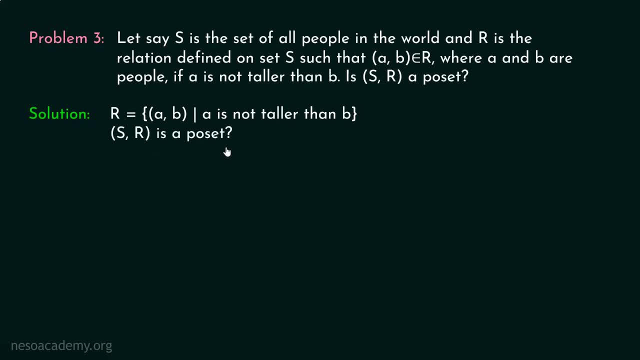 is S, R is opposite. Let's check the reflexive property. According to reflexivity, we must check for all. A belong to S, A, A must belong to R. Is it true that A is not taller than A? Obviously, this is true. 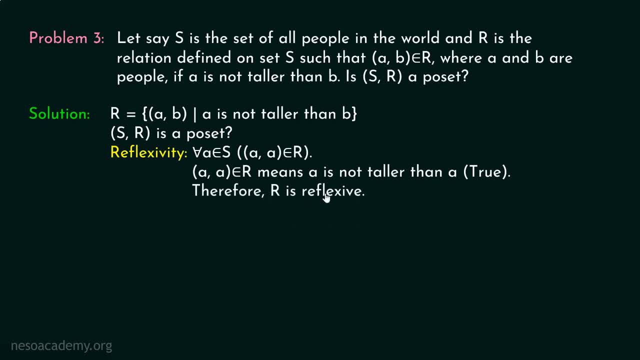 Right. Therefore R is reflexive. This time R is reflexive because here we are saying A is not taller than B. We are saying here that A, A must belong to R, That is, A is not taller than A. Obviously, this is true. 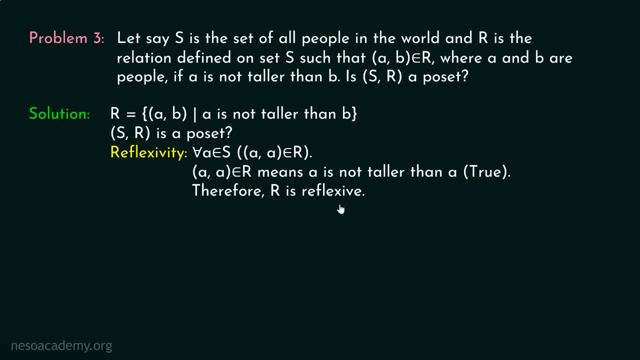 Right. Therefore, this relation, R, is reflexive. Let's see whether this relation is anti-symmetric or not For all. A, B belong to S. if A, B belong to R and B A belong to R, then A is equal to B. This means: 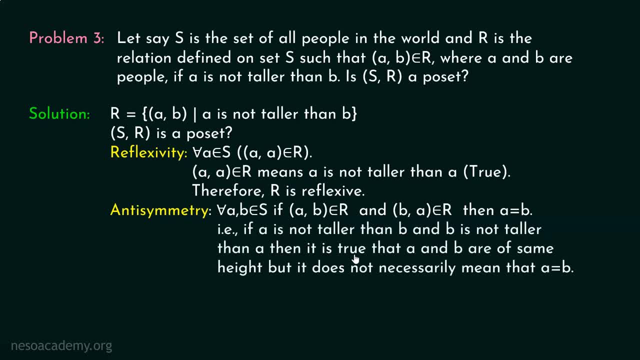 if A is not taller than B and B is not taller than A, then it is true that A and B are of same height. This is what we mean, Right? But it does not necessarily mean that A is equal to B, Right A? 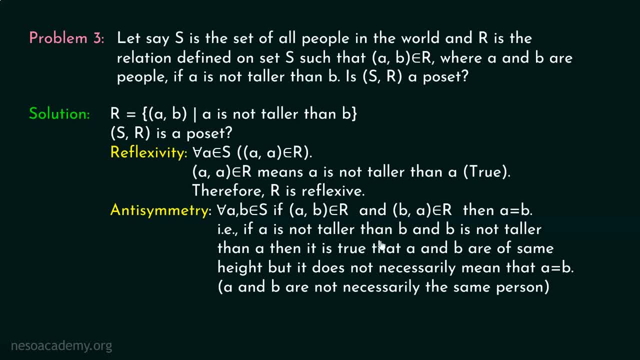 and B are not necessarily the same person. If A is not taller than B and B is not taller than A, then this means A and B are of same height, But it does not necessarily mean that A and B are the same person. Right, Therefore, this: 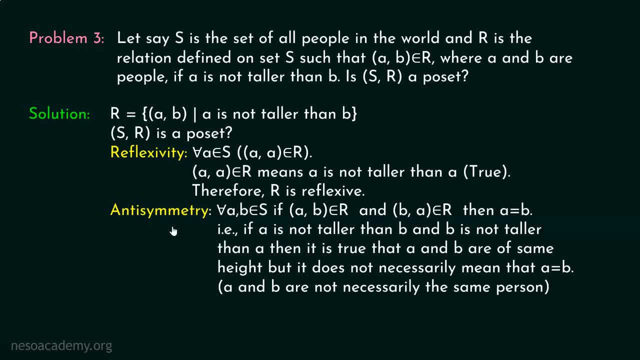 relation, R is not anti-symmetric. Right, You can check the transitive property as well on your own, But it is clear that is not opposite, Because R is not a partial order, And this is true because R is not anti-symmetric.